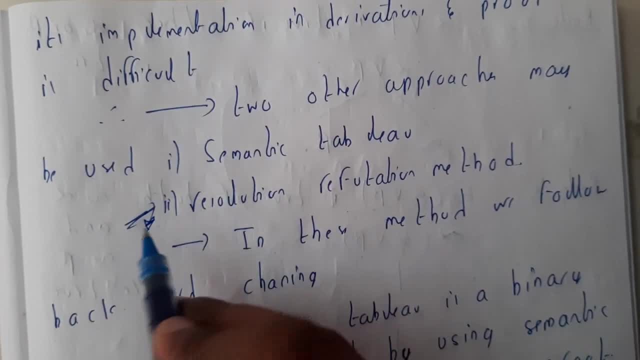 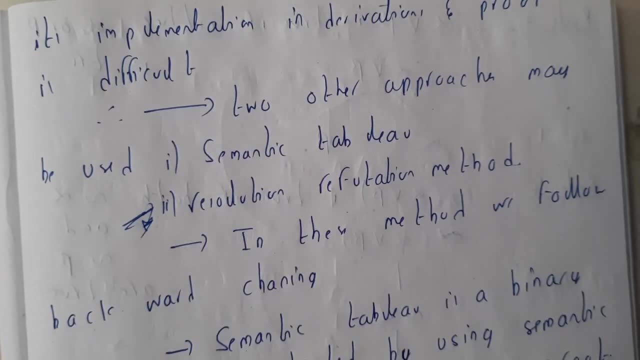 will be discussing in our next lecture. guys, Please don't miss this chapter, this topic, guys, Because in a main resolution topic, you will be discussing about this. So that's the reason why I'm saying please don't miss this topic. Okay, So in this method we follow backward chaining. Yes, 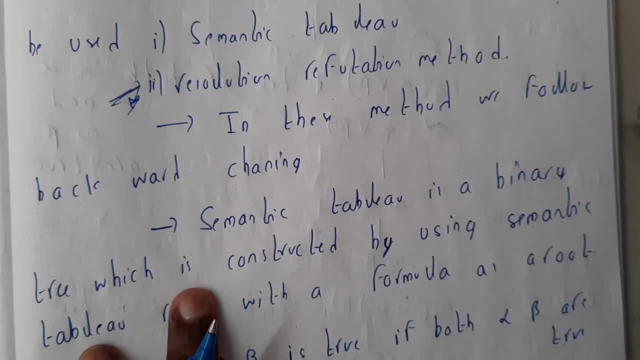 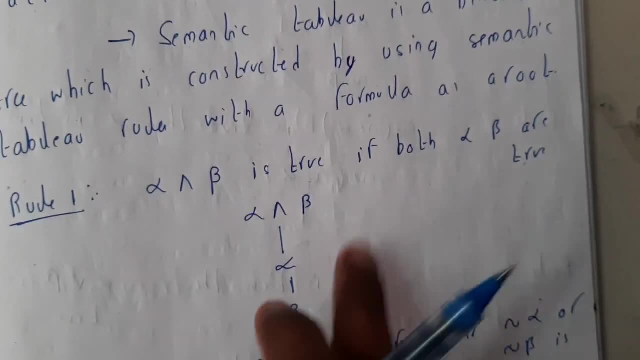 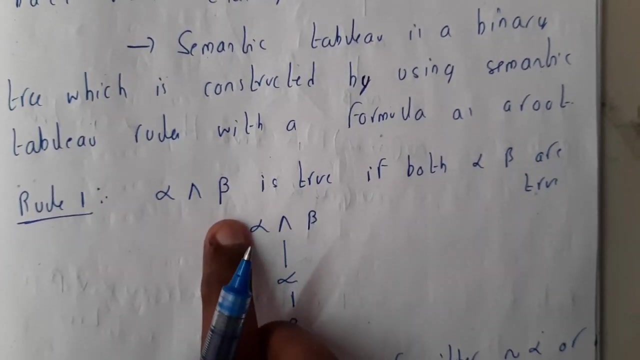 Sematic tabulate is a binary tree, So we will be drawing a binary tree. It is constructed by using the semantic tabulate rules with a formula as a root. So here the formula will be given and we will be deriving a tree for it. Fine, Okay, So if it is alpha and b. So, guys, I'll be just 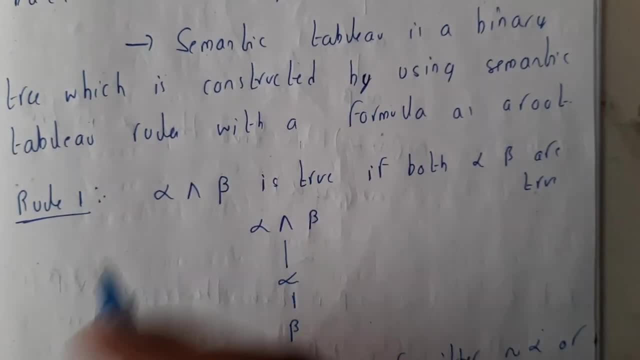 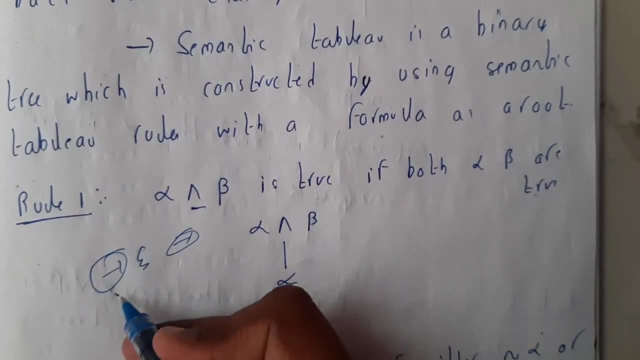 saying you some tricks. Please remember them guys, Please. So and And means if, then this, then right. So you are a. let us take you like pen And pencil. So pen, pencil, you want both. right, You like both. So in that situation you'll be. 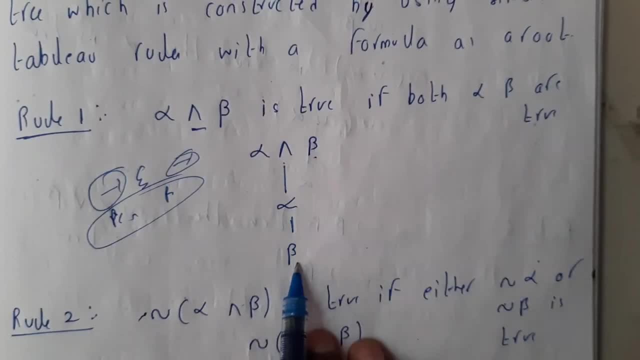 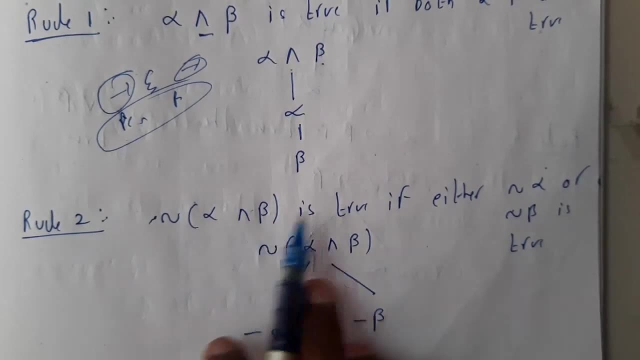 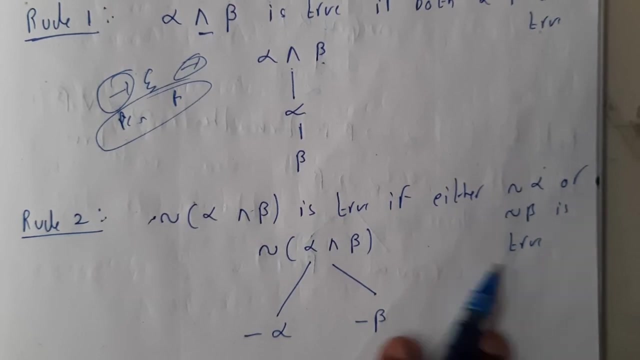 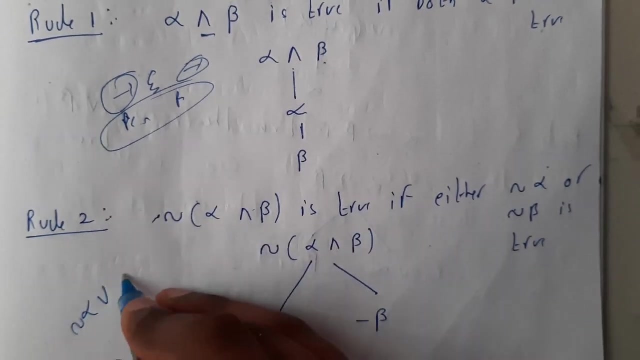 writing one after the other: alpha and beta. So alpha after beta, Okay. So negation of alpha and beta is true. if either or is al, sorry, and alpha or and alpha is true, Okay. So basically, I hope everyone knows the conversion of this to normal. So after, by applying the De Morgan's law, or alpha, 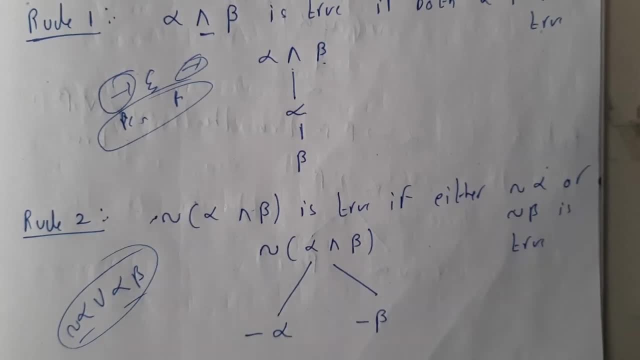 it means to beta. So here both are negative and the symbol in between is or right. So if it is, or I told if it- and it will be writing one after the other. If it is, or you'll be writing one or other. 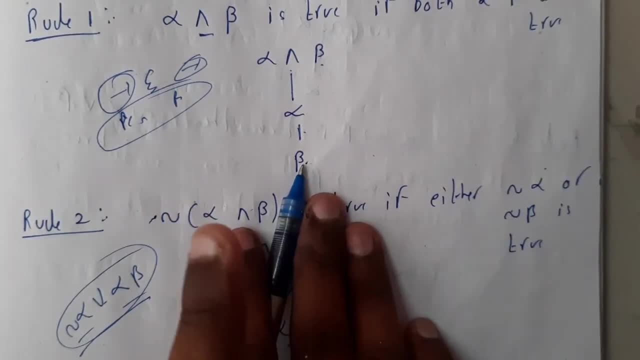 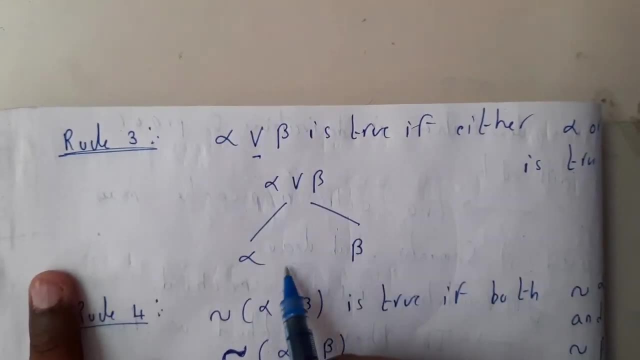 So if you can select this or this here, you need to select both. Understood The logic, that's it. If you know this logic, you can write any statement. guys, It's just a matter of seconds for you to write. So if it is in between or you'll be writing a separately. If it is in this way, do the 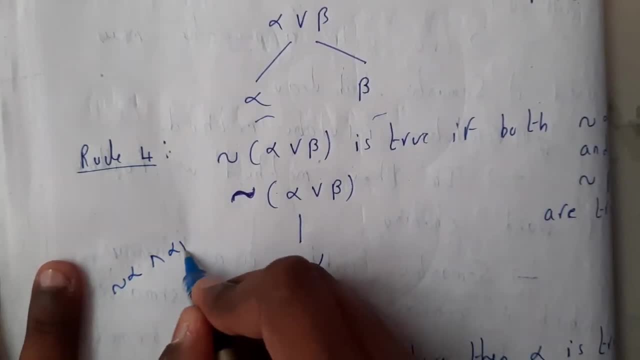 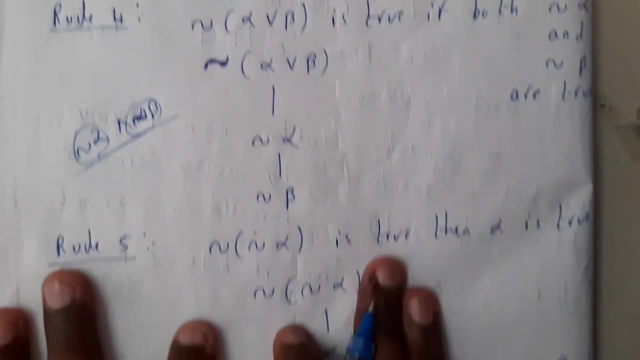 operation And alpha beta. sorry, negation of beta. So if it is in between or you'll be writing beta, So this will this and this are, both are compulsory and means one after the other, Perfect. So negation of negation of alpha is nothing but alpha. So directly, alpha alpha tends to beta. 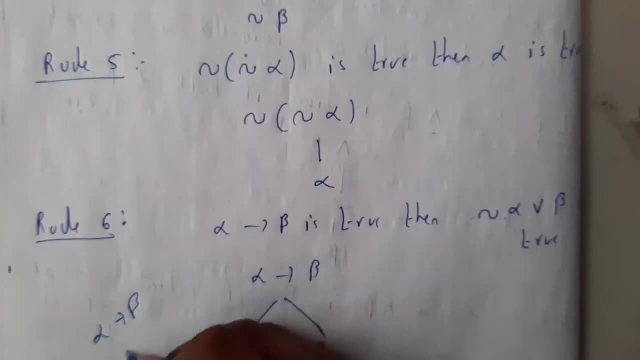 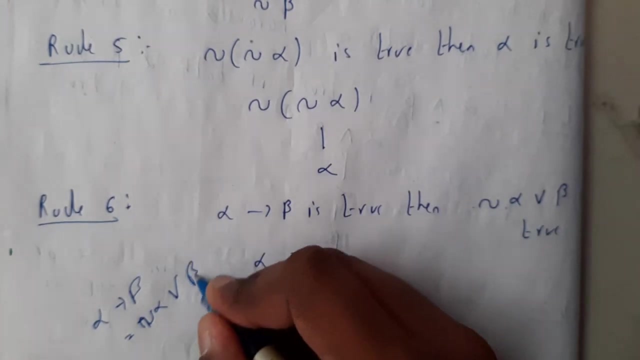 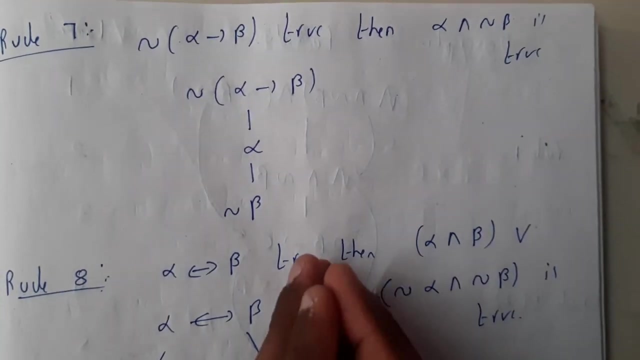 Remember, guys. So I hope everyone knows the formula: alpha tends to beta can be written as negation of alpha, or, sorry, negation of alpha or beta or B. So in this way you'll be writing in between, or so you'll be writing, or, Guys, just by the small trick which I have just told you. 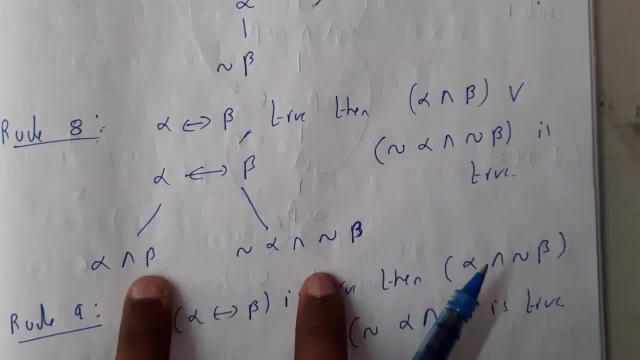 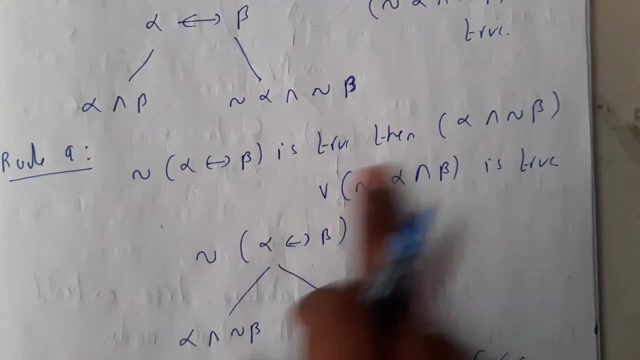 you'll be applying that. That's it. So similarly for this, also for double implies you'll have two different. I hope everyone remembers that. So even if you want, you can further divide this also. guys like branches, Fine, Okay. So similarly for 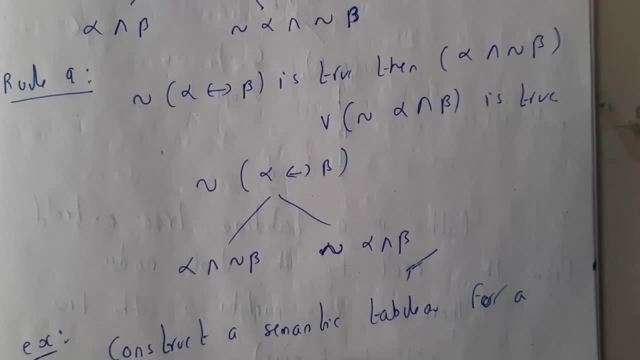 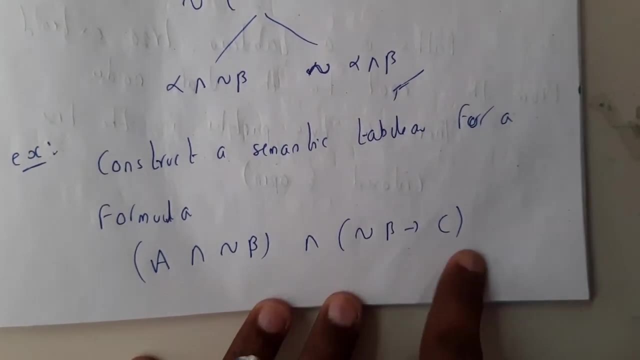 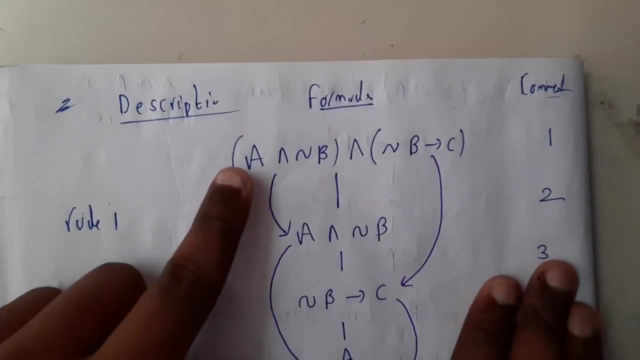 double implication on negation also same. So I hope everyone got a small idea on this. So now let us go through a small problem so that you'll be having a clear idea. So the given question is this: So he asked us to reduce that into a graph, Okay, Okay. So initially let us take this and 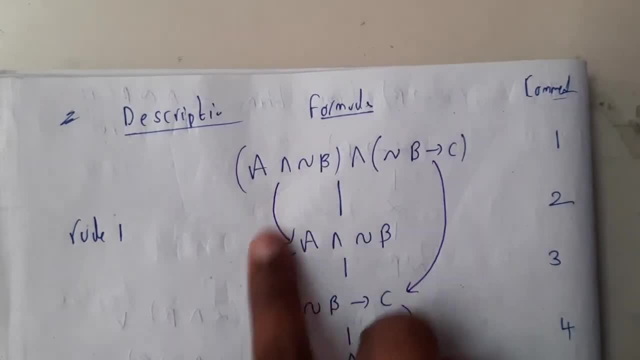 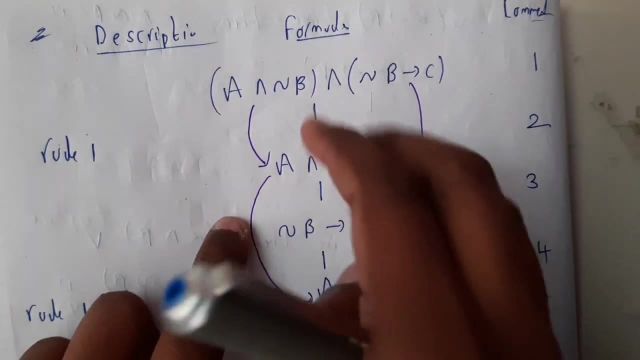 this guys. So this as one, this as two. So I took this whole part here and I took this whole part here. So in between and right So, and means one after the other. So here I wrote this, here I wrote this, one after the other. So now we 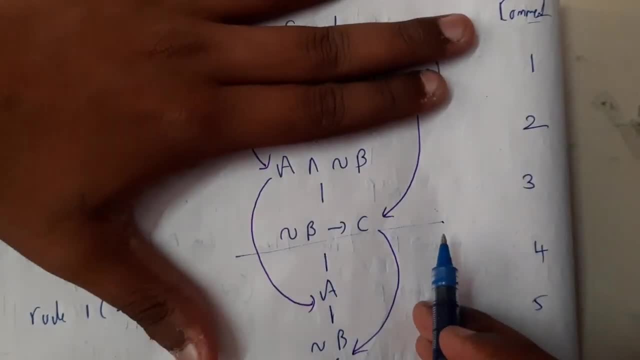 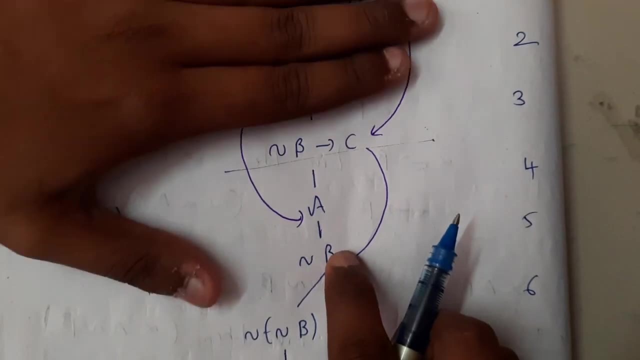 are done till here. So now these two application is over. So just to close them. So now come from here. So here the between symbol is and: So this after this, So A after B. Okay, So now we are done with this also. So after this you need to do this. So negation of B. So exactly, it is starting. 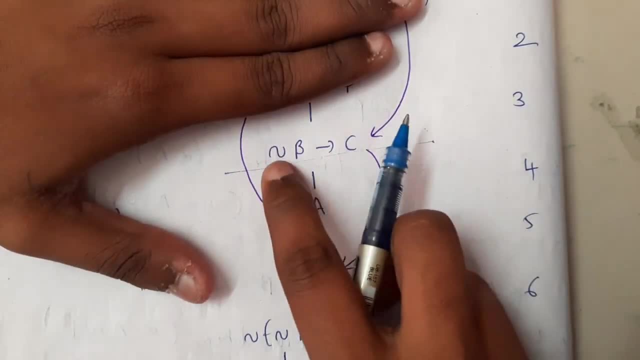 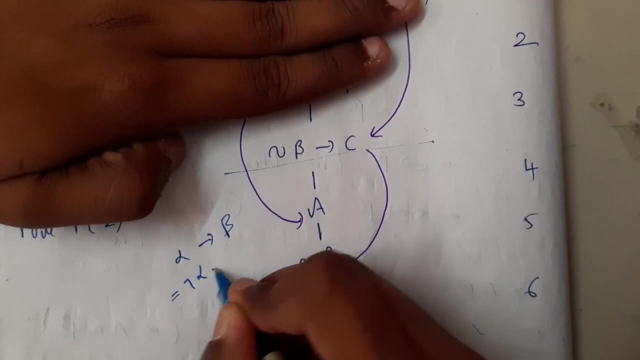 here, right? So connect them. So, negation of B: you need to get a. negation of B. tends to C. So I told you, tends means alpha, tends to beta means what I told guys: Negation of alpha or beta- right? So this we will be applying. So, negation of negation of B or C: So now we are. 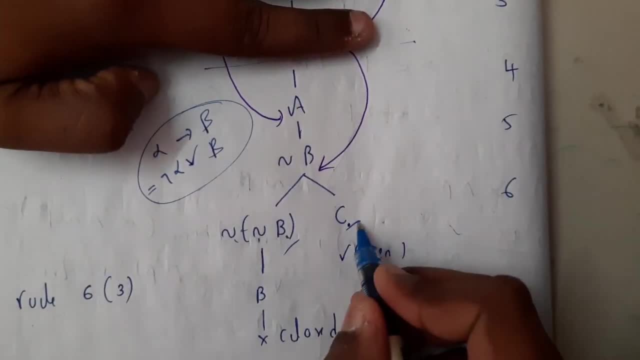 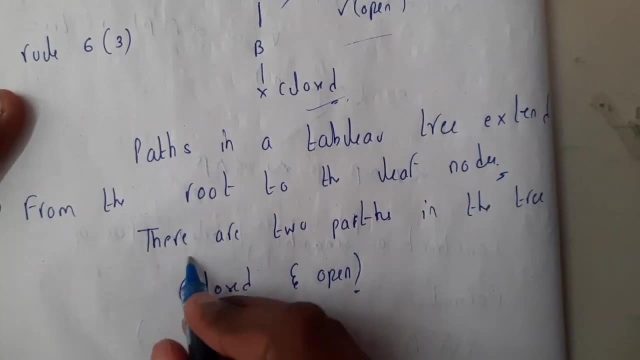 done till here. So is there any further amplification till here? No, So this is closed and this is also closed. So this is the path, guys. So path in tabular tree extends from the root to the leaves. So there are two paths Those are nothing but closed and open. Okay, So I hope. 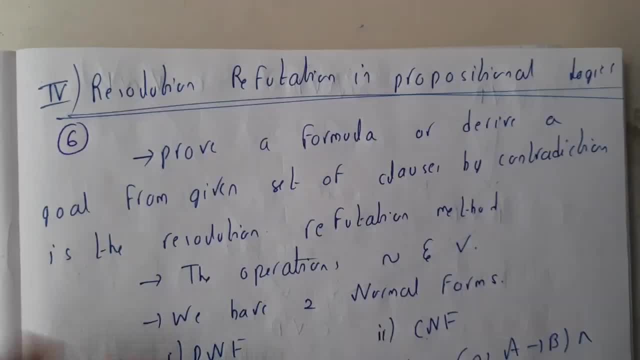 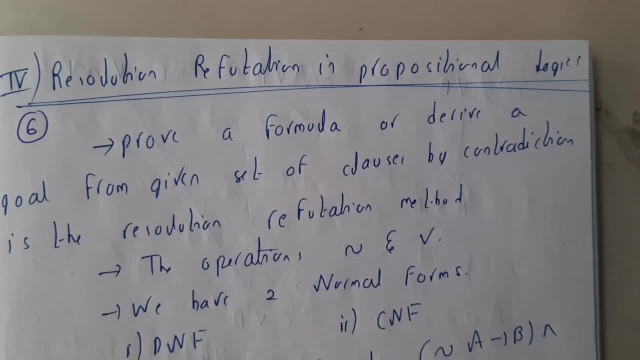 everyone got a clear idea on this, So in the next lecture we'll be going to talk about the resolution reflation in propositional logic. Guys, this topic is again covered in first order, predicate logic or predicate logic, So that's the reason why I'm just forcing you to watch. 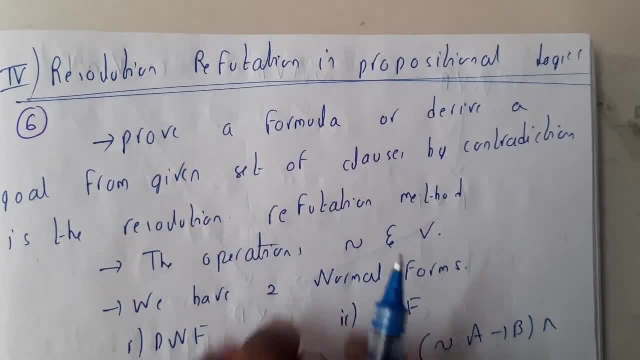 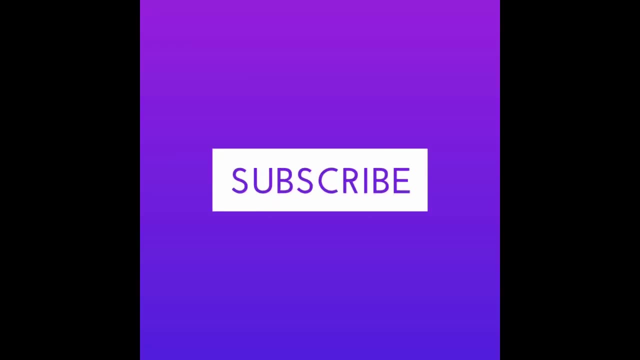 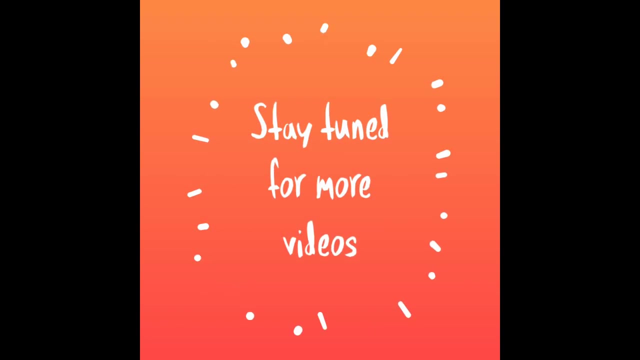 this lecture, guys, please, Because there is a 10 marks question completely based on this concept. almost So, let us meet in the next tutorial, Thank you. Thanks for watching, Bye.